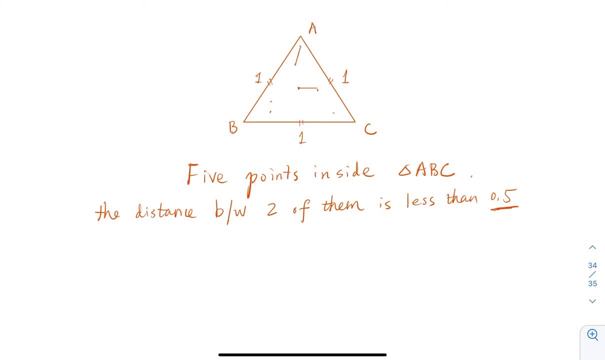 Now, however, here we want to show that if you get any 5 points right, you can put random points here Here. sorry about that. Let's try to 5 points here. you know, let me see 1 point here right, 1 point, 2 point here. here you can put them as far as possible. but then you know, if you add more points, some points have to be close to each other. 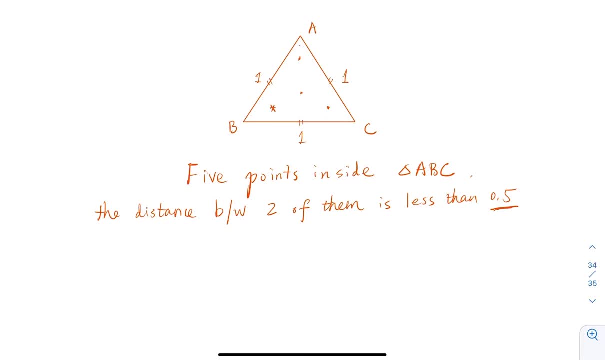 So right now I have 4 points, but if I add the 5th point, I don't know, no matter where I add, it cannot be too far away from others, right, If you can try to add it here, You know. but maybe you know some of it must be less than 1 half. 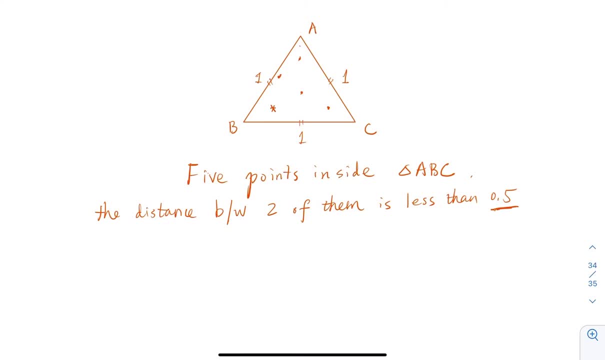 How do we prove that? Why don't you think about it? You could pause the video if you want to. Now let's review the answer. So notice that we have 5 points right And we want to prove it's less than 0.5.. 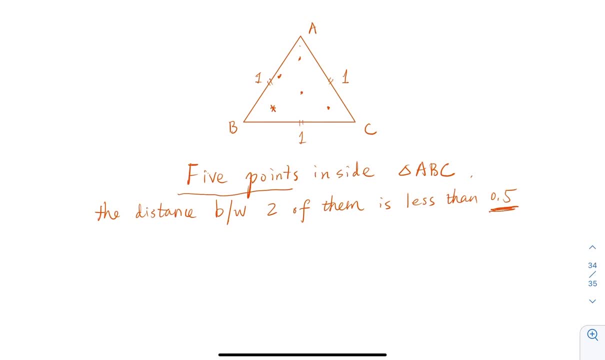 For the equilateral triangle, right For the equilateral triangle, right For the equilateral triangle. we can subdivide the triangle into 4 equal areas, right? So if she gets the midpoint here right And get the midpoint, you connect them together. 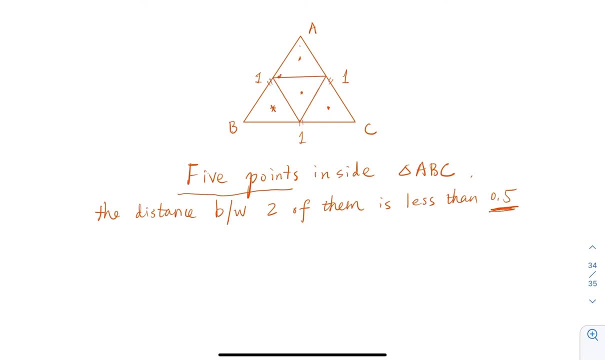 We can prove that all the triangles here are congruent with each other And they are equilateral triangles with the side lengths of 1 half. And they are equilateral triangles with the side lengths of 1 half. So we subdivide, you know. 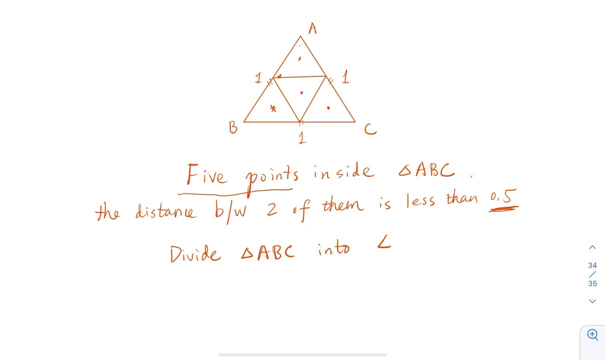 a- b- c into 4 equal parts: right a- b- c into 4 equal parts. right a- b- c. into 4 equal parts. right, And each of which is an equal, And each of which is an equal.